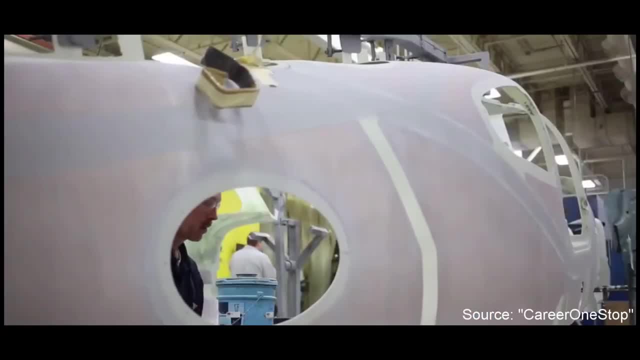 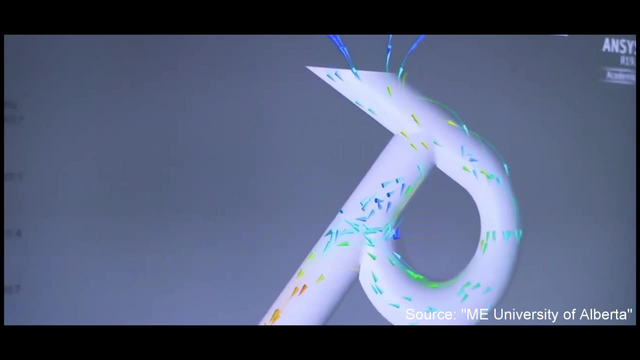 In this video, we will be presenting and explaining many theoretical concepts linked to aerodynamics and, more generally, fluid dynamics, as these two areas of study are fundamental for any aspiring engineer in the aviation sector. Aerodynamics is the study of the forces and motions of an object or body passing through 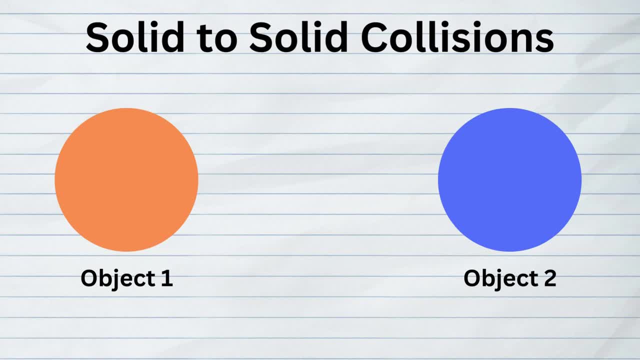 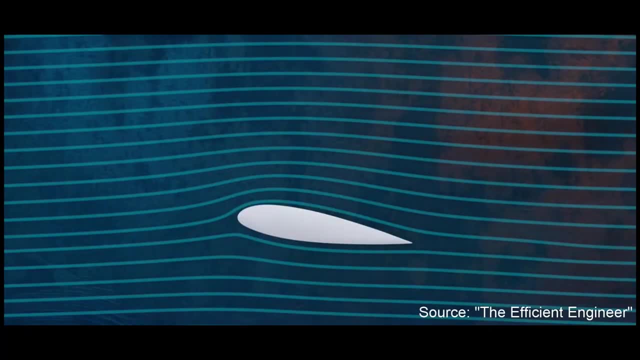 the air. When two solid objects collide, they do so by transmitting forces through the points of contact. This is not the case when a solid interacts with a fluid due to the air being able to change its shape and wrap itself around the object. Due to this, the mechanical forces 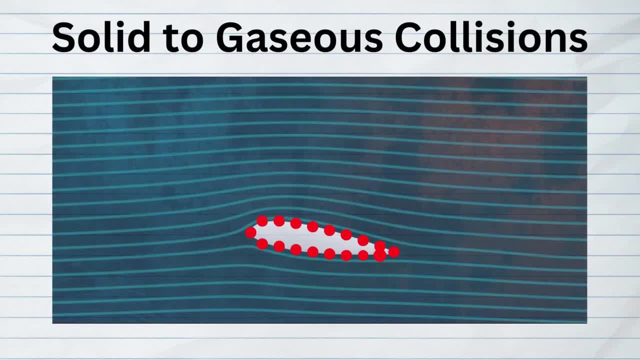 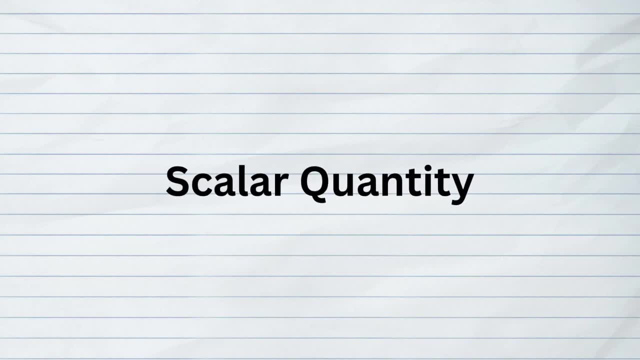 that result from the interaction between solid and gaseous substances occur at every point along the object's surface and not in a singular location. This happens because of the fluid's pressure. Pressure is a scalar quantity, meaning that it does not have a direction, but only a. 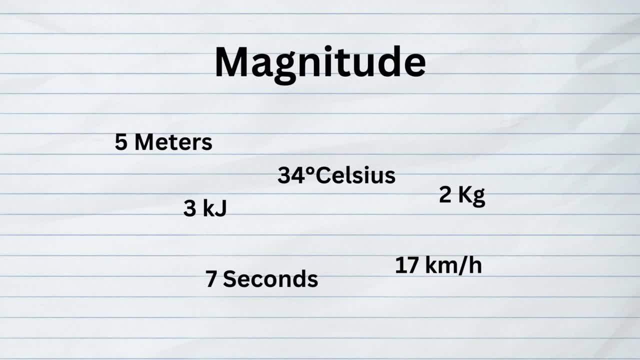 magnitude or size. Pressure is, in this case, related to the momentum of molecules in a fluid and can be defined as being equivalent to the force applied on an object divided by the area of the surface. Pressure is always perpendicular to an exact point along an object. 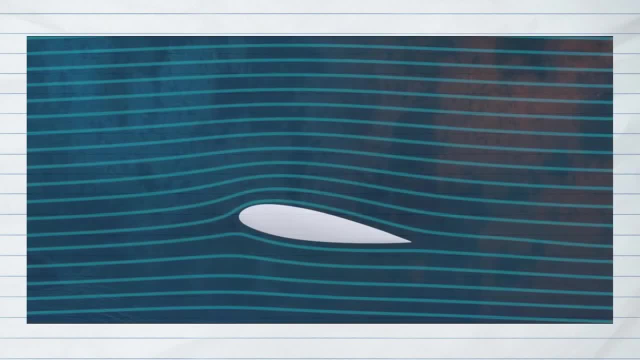 Let's take an airfoil as an example of a body affected by pressure. This object has a particular teardrop-like shape as it allows it to generate great quantities of lift, of which we will be discussing in more detail later on. If we were to take the cross, 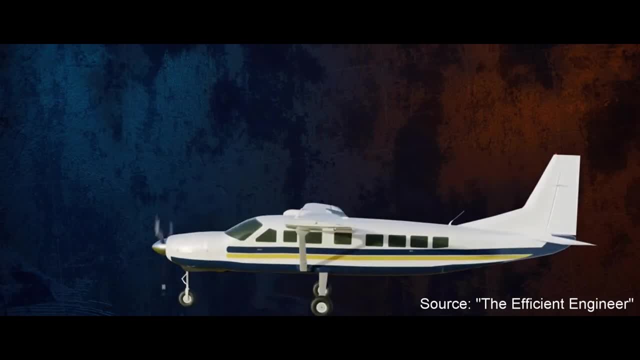 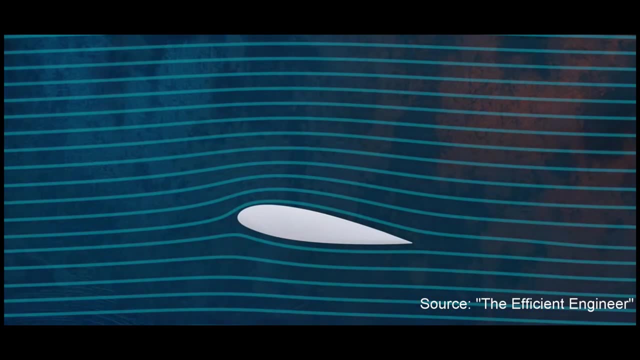 section of a plane's wing. we would notice this characteristic shape also used on sails and propeller blades. When an airfoil flies through the air, it is influenced by the fluid's pressure in different amounts depending on the location, For instance, the top and bottom of the airfoil. 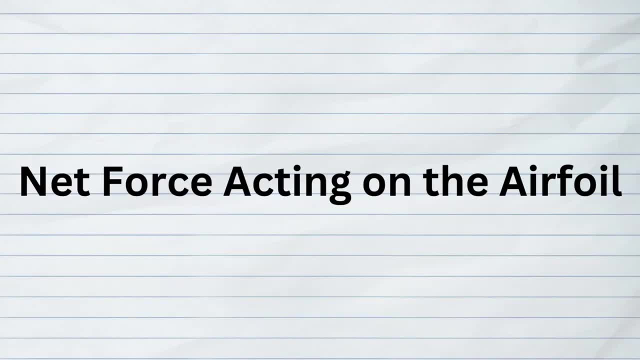 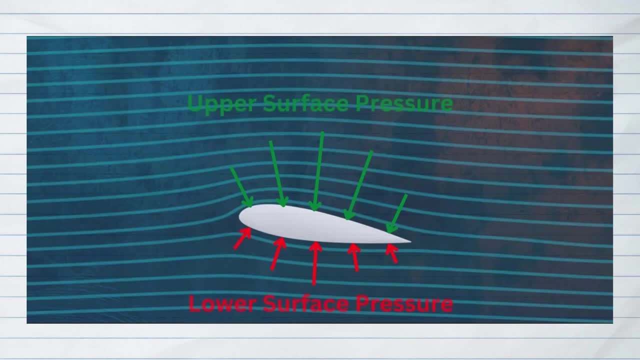 won't be affected by the same pressure as with the front and rear. The total force acting on the airfoil is calculated as the sum of the pressure on all of the infinitely small points of the body's surface. If the pressure is the same along the entire airfoil, then no net force is. 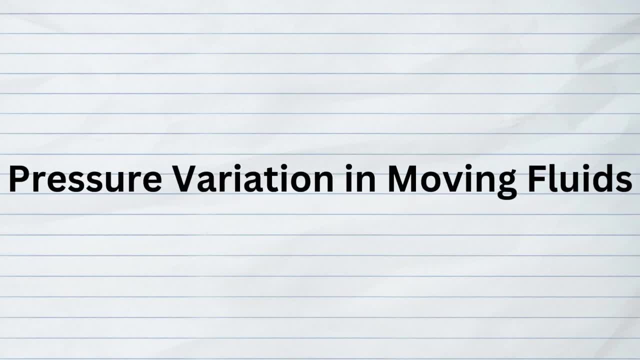 produced. However, if the fluid is in motion, the velocity of the molecules would differ while passing along the airfoil Due to pressure. depending on fluid velocity, it would vary along the surface of the airfoil, creating a net force. The fluid's direction can be defined along. 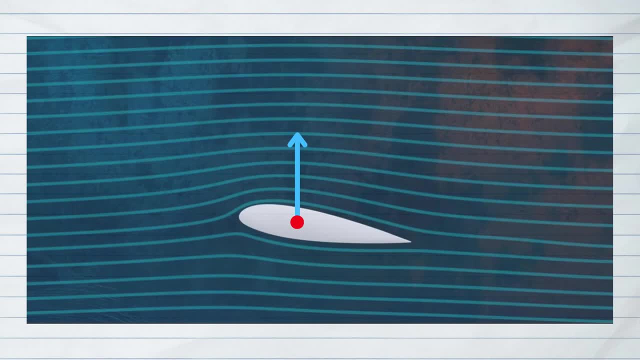 the motion. The component perpendicular to the flow is called lift and is essentially what lifts the airplane, caused by the difference in pressure along the airfoil. The component that acts in the same direction as the fluid is drag, which is the resistance that the airfoil 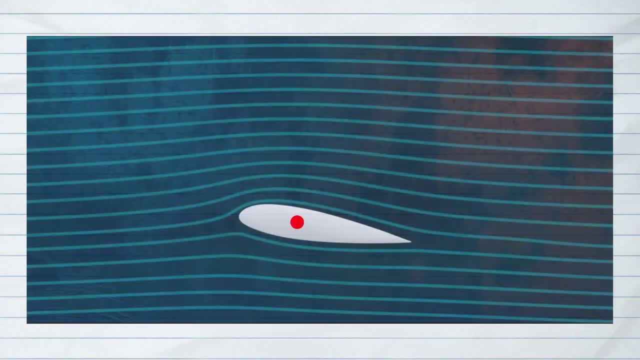 encounters when passing through the air Observing an airfoil. the center of pressure is the average force that acts along this body while passing through the average point of the object. The center of pressure is also the point in which the net aerodynamic force acts from. 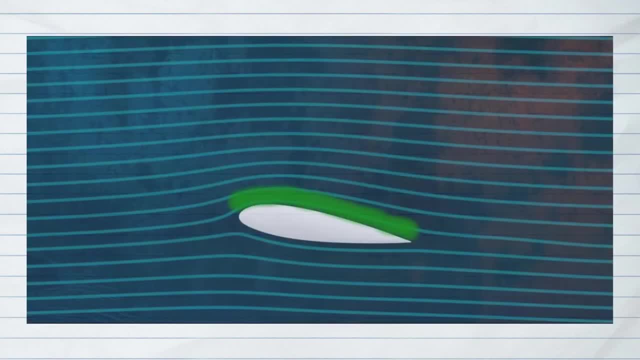 In a standard airfoil, the velocity of the fluid is greater when passing along the upper surface and smaller when passing along the lower surface. This means that the bottom has a greater pressure compared to the top, creating lift. The difference in pressure along an airfoil causes torque. 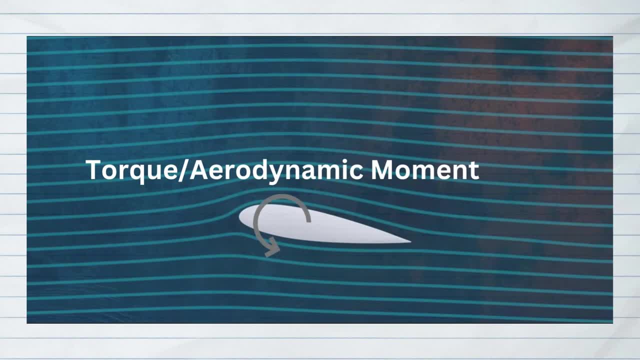 also known in this case as aerodynamic moment, which would cause the wing to flip if not restrained correctly. The point along this body where the moment remains constant is called the aerodynamic center and is much more accurate than the center of pressure in determining. 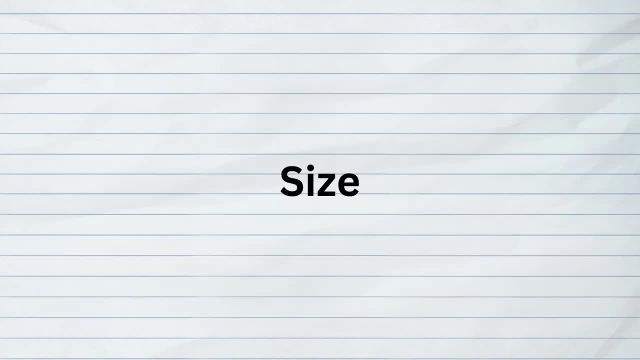 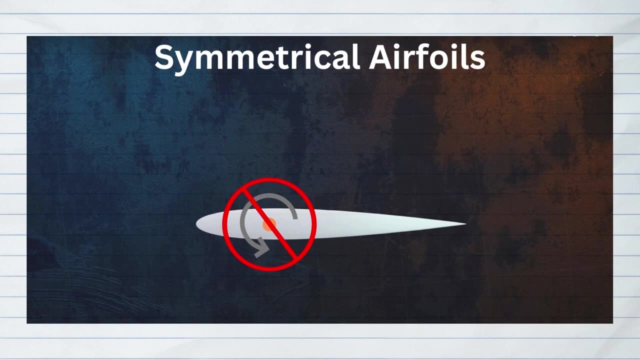 aerodynamic behavior. Depending on the wing, which differs by shape, size and thickness, the aerodynamic center can have varying characteristics. For example, symmetrical airfoils have no torque around the center for all angles at which the fluid meets the airfoil. 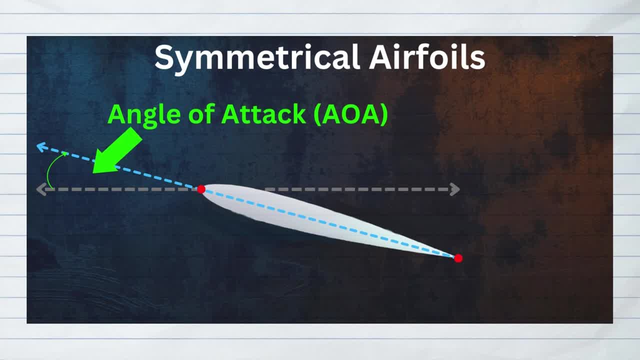 also known as the angle of attack. Wings that are curved or cambered have a torque and in some cases, this moment can vary with angle of attack. After considering the aerodynamic center, it is important to know that the center of the aerodynamic 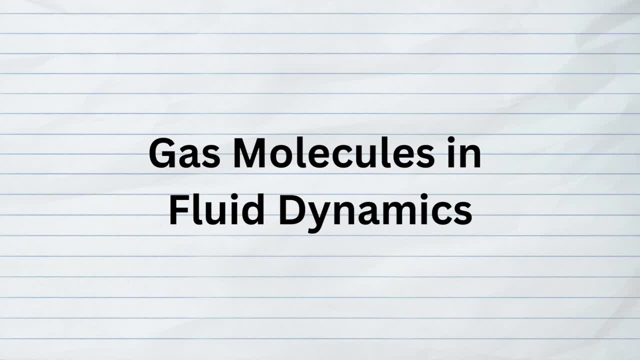 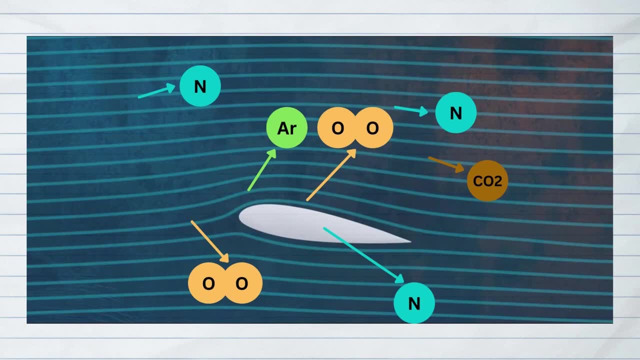 the implications of pressure. we can look into the effect that gas molecules have on airfoils. The atmosphere is formed by many gaseous elements which are disrupted when an object passes through them. This penetration of the air causes aerodynamic forces to be produced which depend 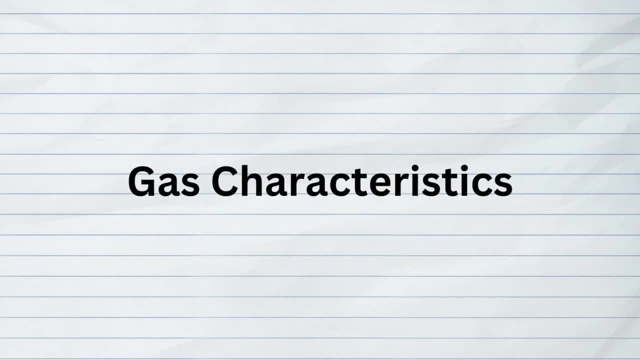 in magnitude, on the shape and speed of the airfoil, as well as the characteristics of the gases. There are three main features that all gases have, being viscosity, or the stickiness of the gas, compressibility or the springiness of the gas, and density, which is a measure of the compactness. 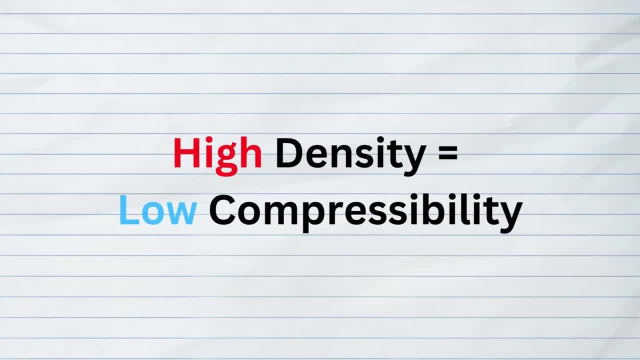 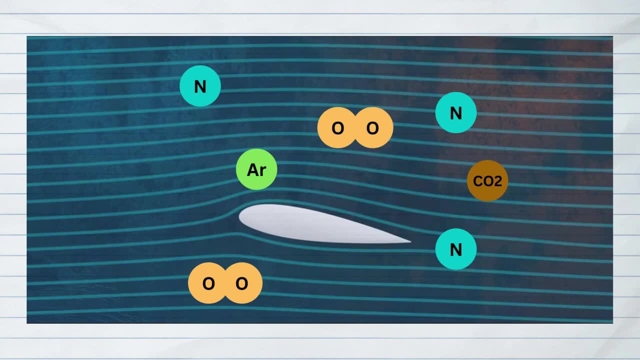 of a substance. Usually, a higher density of the gas will lead to a lesser compressibility, and vice versa. In order to better understand how these characteristics influence the aerodynamics of an airfoil, aerospace engineers use similarity parameters which compute ratios between external 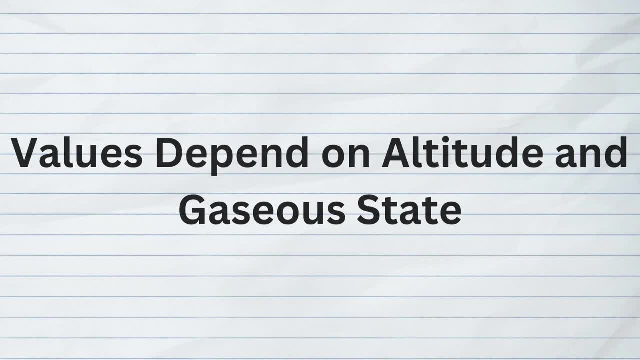 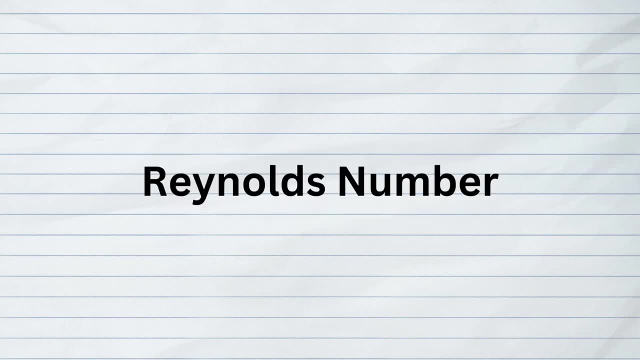 forces and those generated by the features of the gases. The values of these parameters depend greatly on the altitude and state of the gases, which both have pronounced effects. An important similarity parameter is called Reynolds number and focuses on the relationship between gaseous forces generated by the gases. 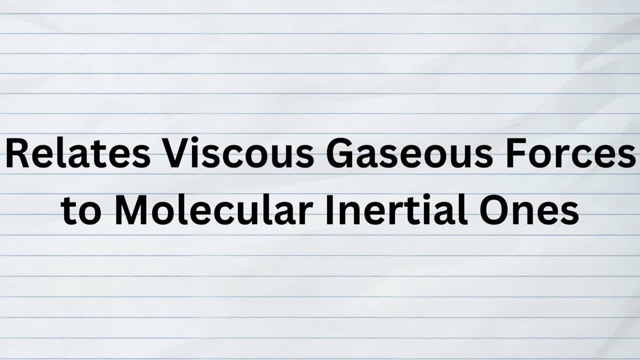 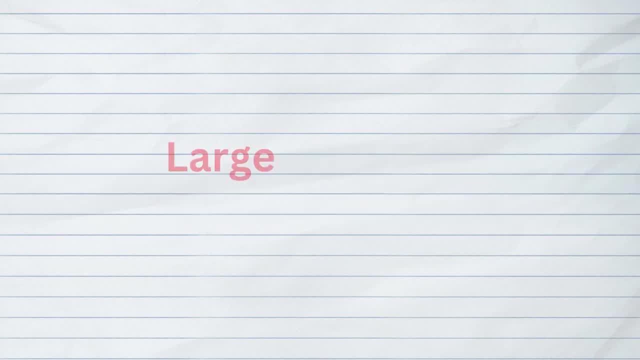 This number is dimensionless, meaning that it is not associated with any unit of measurement, and can range from 100 to 10 million, with larger values signifying lesser viscous forces. The boundary layer is a phenomenon caused by the viscosity of gases and affects the aerodynamics.